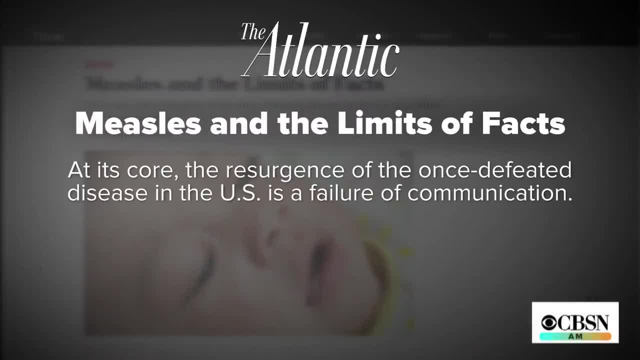 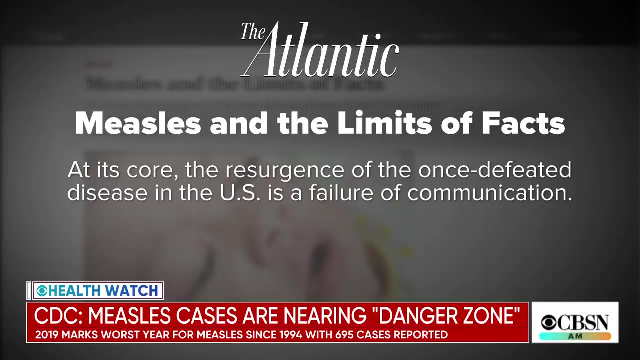 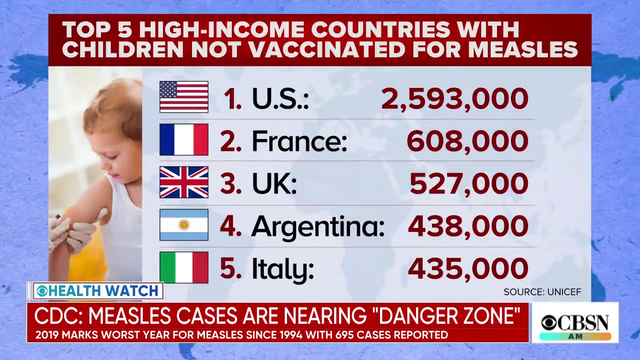 So, doctor, why is the United States having such a hard time controlling the spread of measles? A lot of it comes back to information, misinformation, misconceptions and actually considered disinformation campaigns where people misunderstand the risks and benefits. And it's complex. People have different relationships to the medical system And also your, your perception of risk sort of wanes over time when you forget that measles is an, is an actual 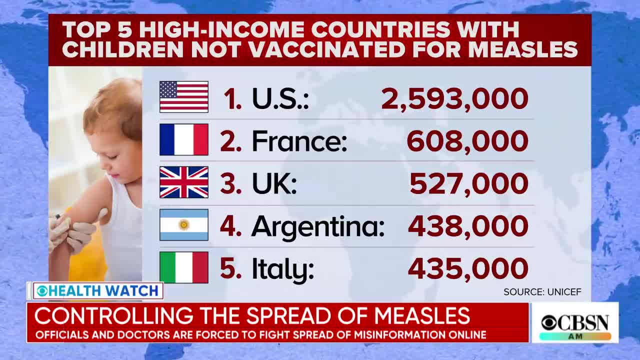 deadly disease. It becomes easier to become susceptible to thinking about harms of vaccines as minimal and almost non-existent as they are. I'm not sure if you know the answer to this question, but we just read out. you know some statistics saying that so far this is the sort of the worst year since 1994, 1994, 963 cases. Do you know what happened in 1994? Now, as I understand it, we're just a, you know, a few months into, maybe almost halfway through this year, and we're already at 695.. So who knows where we're going to end up. 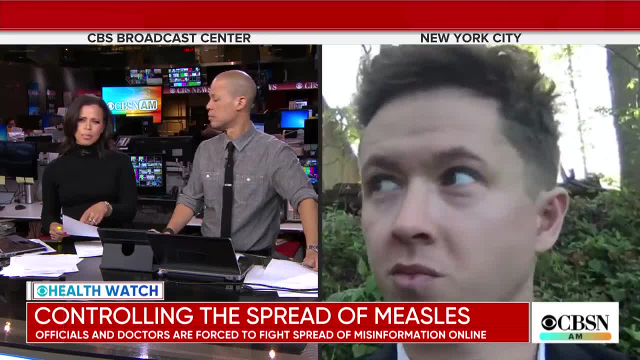 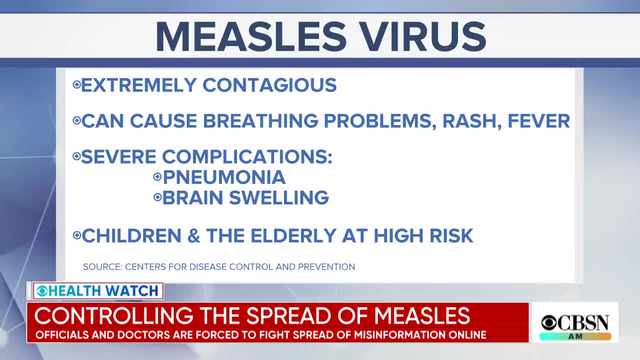 At the end of the year, But what's up with 1994 being a bad year for measles? I don't recall, Just just sort of I'm sorry. It was generally, though, that it was on the decline from the 80s and 90s until 2000.. And there were some outlier outbreaks, as there are with any infectious disease, But generally there was a real good line of progress over the course of decades, And for a number of reasons, 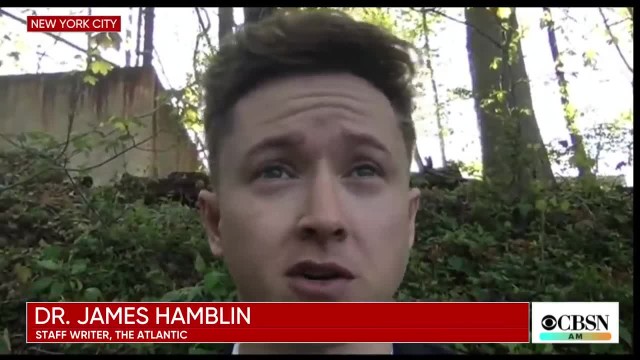 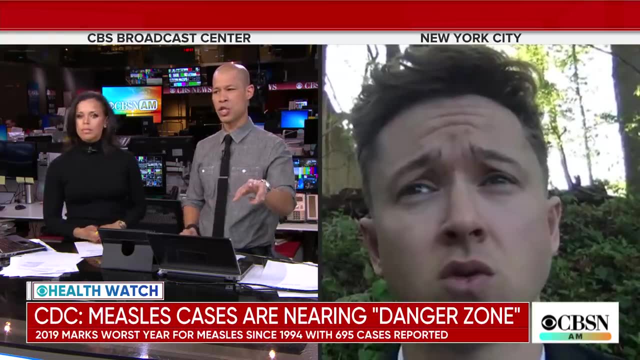 We're. we're going back in the opposite direction, which is the general really concerning. So it's interesting to me too, Dr Ann Marie, because I noted the countries that we just showed on that graphic there that are leading the world in number of measles cases reported: the United States, the UK, France, Italy. 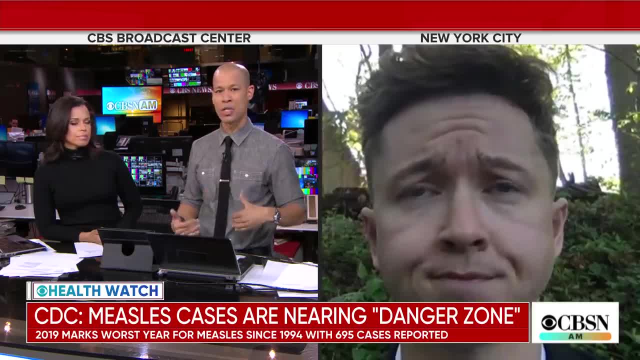 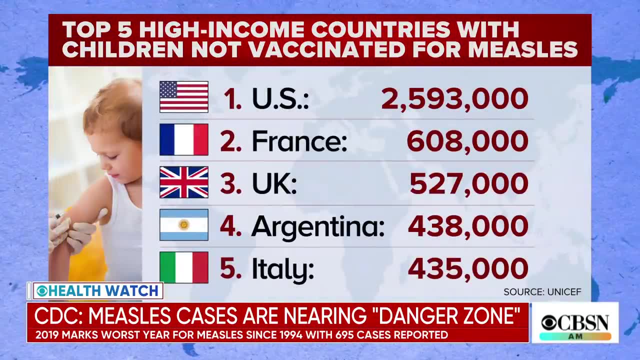 I didn't see Canada on that list, interestingly enough, And I remember as a child getting vaccinated for measles, MMR. It was just the thing that you did. You're you're, you know you would. you would start school and your parents would say you got to get these vaccines, or the school nurse. 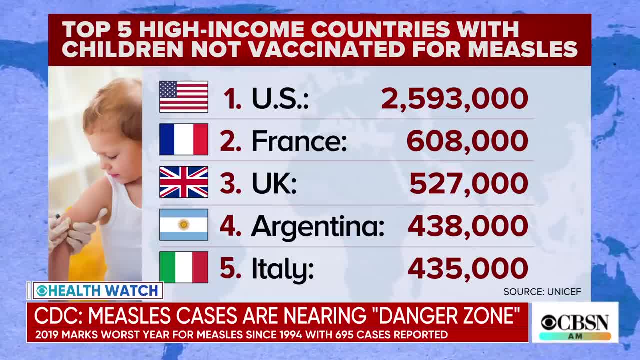 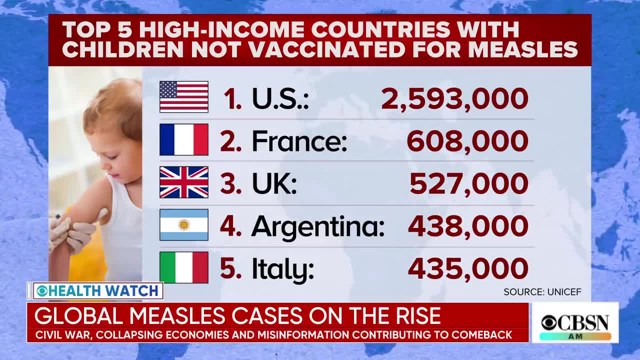 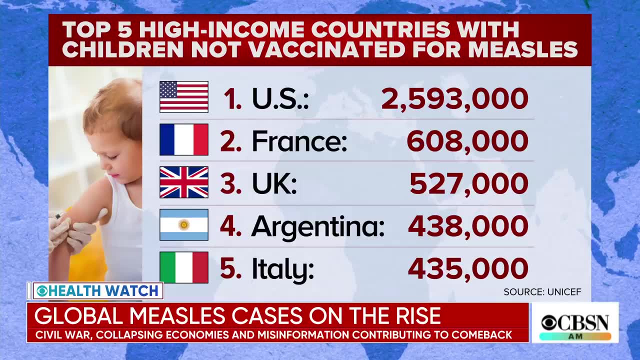 Would say: you got to get these vaccines. And I just- I've gone back to this repeatedly when we covered this story, doctor, which is that I've worked and reported from countries, a lot of third world countries, where thousands, if not hundreds of thousands, of people have been affected by horrific diseases that have been eradicated in the United States and in first world countries. 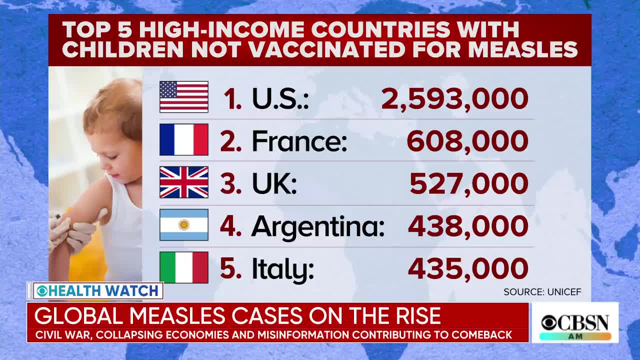 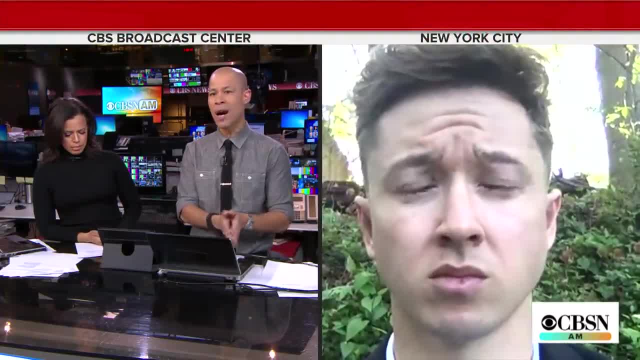 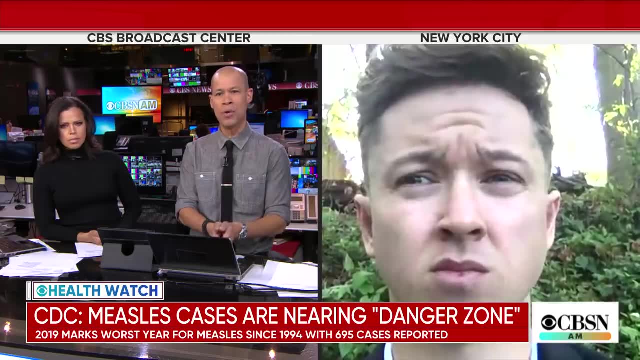 And when you see a country like the United States taking a step back, and when you talk to families in other countries where they don't have readily available vaccinations for their children, and they just look at us and they wonder, they scratch their heads and say how, how, how, if you have this available to your children, to your people, are you not ensuring that everybody is protected? 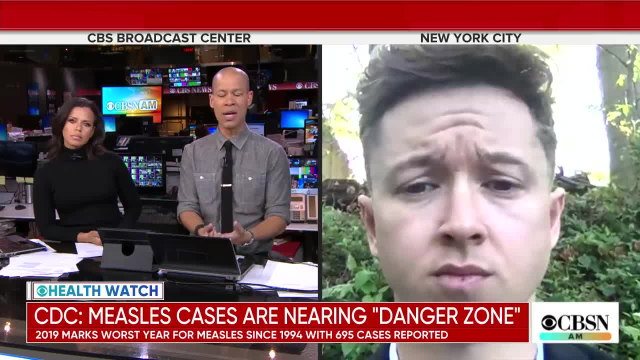 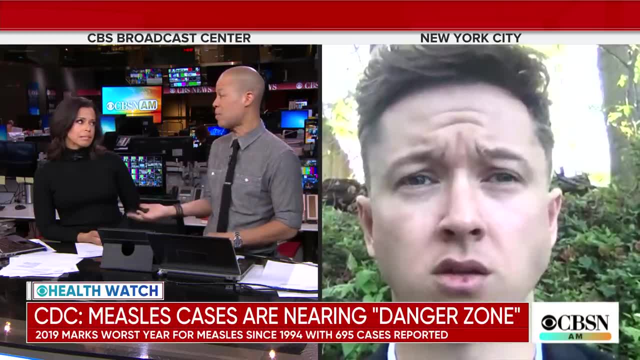 Worse, we would give anything to have the kind of medical technology that's available to you in the US. So it just is sort of boggling to me- And I know that Canada is not on there, Ann Marie, because I'm guessing you're not having that same problem that you have in the United States. 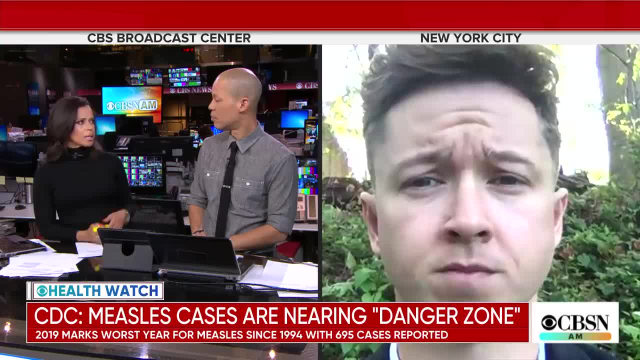 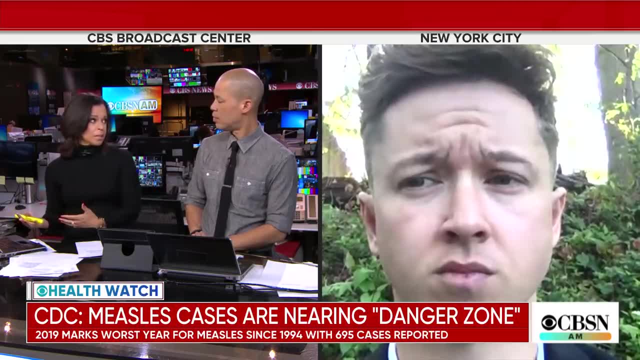 I saw that too And I at first I thought about the public health care system. But France has a public health care system, So does the UK, And you know you would think that the government would be particularly proactive if they had to foot the bill. 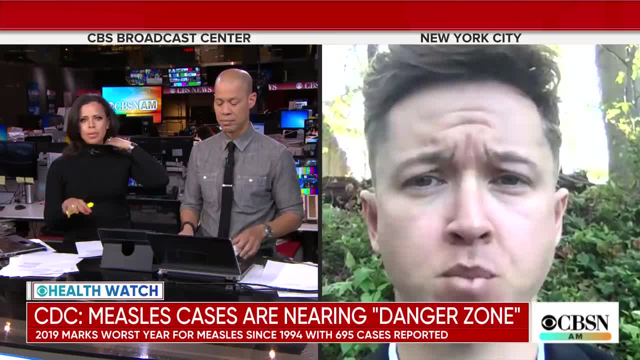 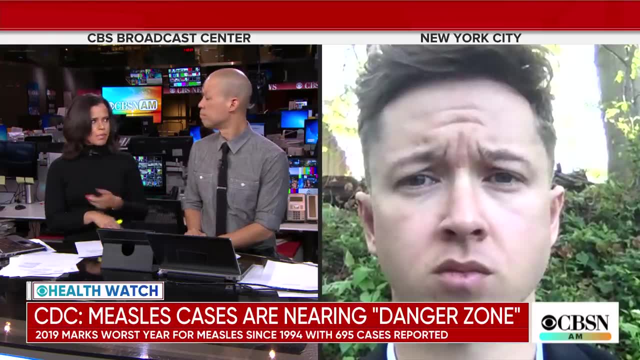 Right, So I can't- even I can't- say what the difference is, But but I'm curious. you know we're looking at a list of countries that are, you know, where access to information is at the fingertips of everyone. You know great education, But this is not just happening here. 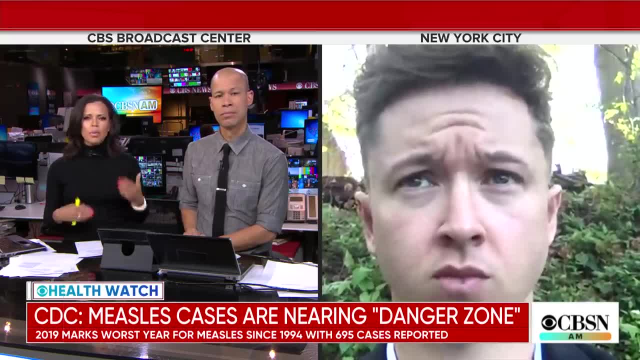 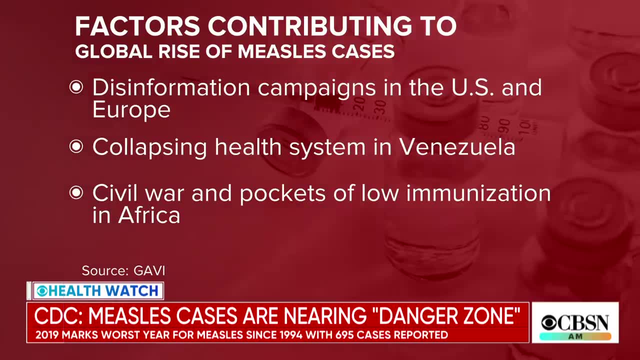 It's happening in other countries. What, what, what's going on? This is a global phenomenon, phenomenon of misinformation. Is that what it is? It is global And that was what's really concerning. The World Health Organization announced this month that numbers are up 300 percent over the same period last year, globally. 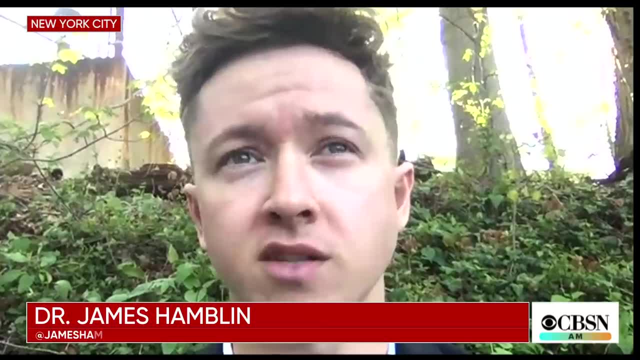 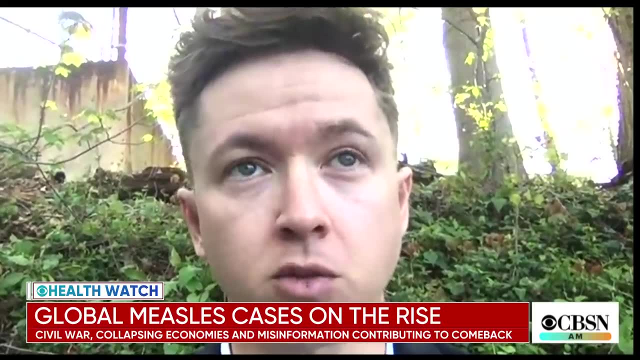 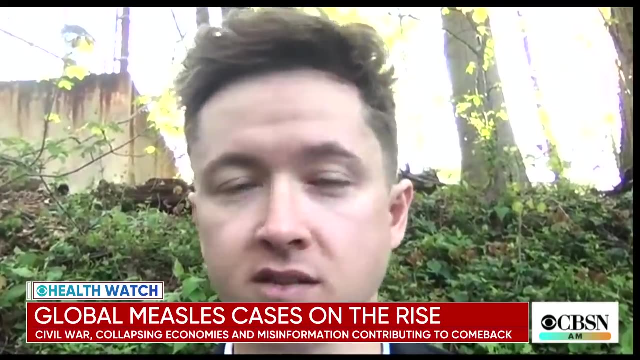 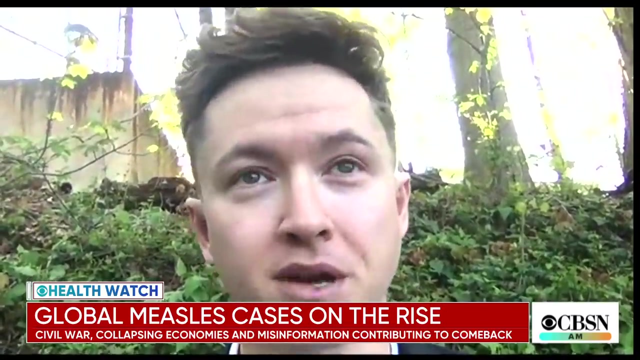 And one hundred and ten thousand people died of measles in 2017.. So, as significant as this is in the United States, it's a much bigger problem globally And the pockets of disinformation that are escalating And the people that are emanating from places like the United States, where it's not a huge problem, are are having effects in places where it has long been a big problem and continues to be. 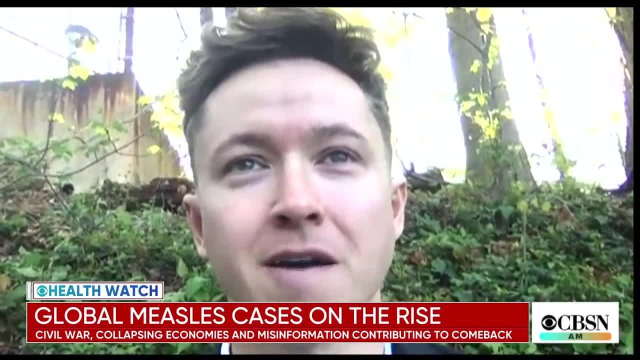 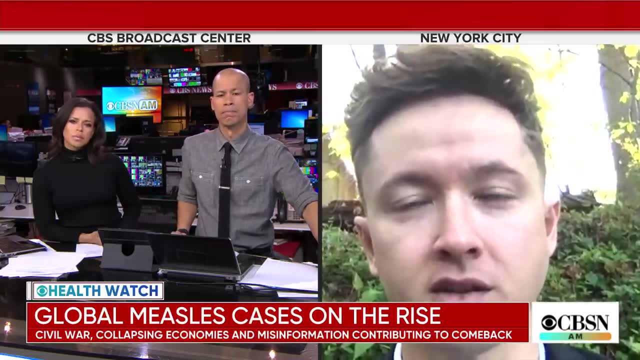 So it is. this requires a global approach- and we're all in this together- And the spirit of understanding that infectious disease is not an individual battle. It's about communities. Yeah Well, we've done interviews on how you know misinformation coming out of the US. 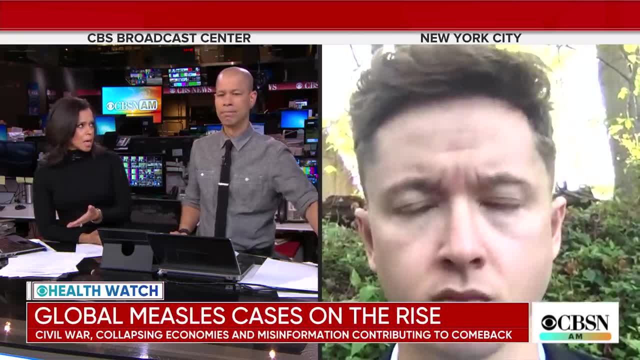 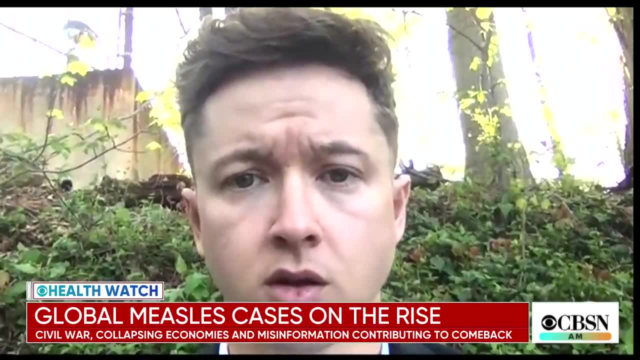 various platforms like Snapchat are making their way to India, where you know an outbreak can be absolutely devastating. It still boggles the mind. It's disconcerting, Dr James Hamlin. thank you, sir, for being with us. We appreciate it. Thank you for having me. 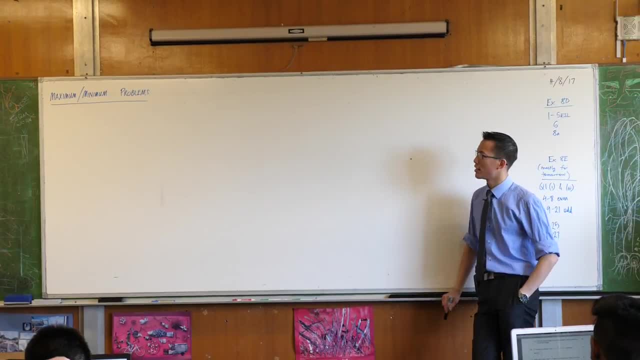 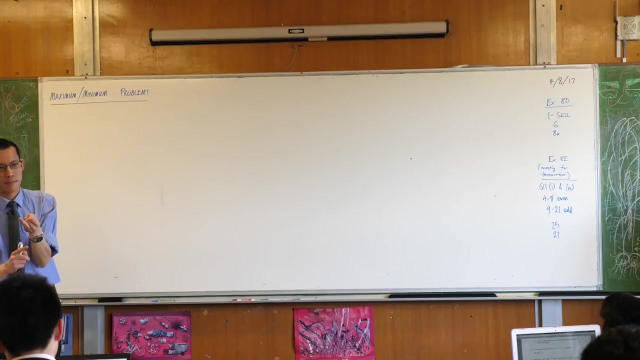 Maximum-minimum problems- which sounds like a bad tongue twister, which is why we call them max-min problems- are a really important category of problem in mathematics because they're so practical. Often we're trying to maximise something, get the most profit, get the most people on the buses. 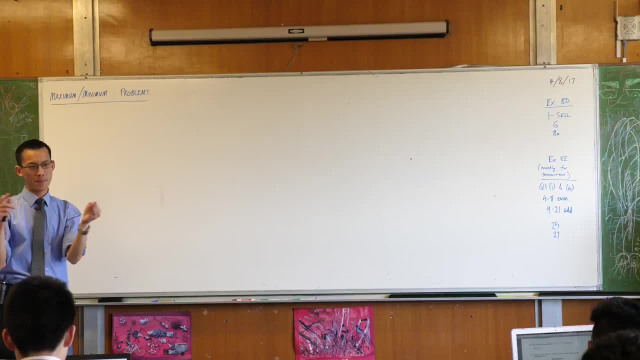 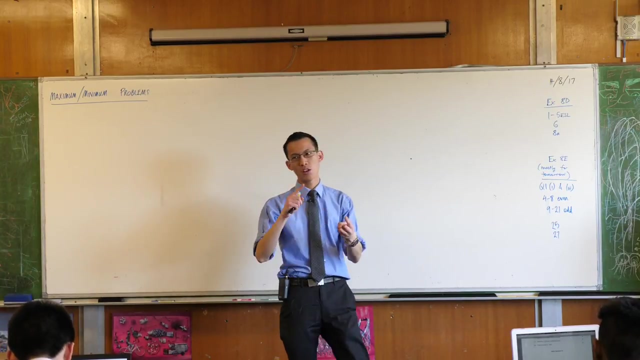 get the largest amount of population in a particular area, so you don't make it bad on resources. and what have you Maximise some quantity or likewise minimise something. Can you get the lowest cost? Can you get the lowest greenhouse emissions? Can you get the lowest fuel consumption? 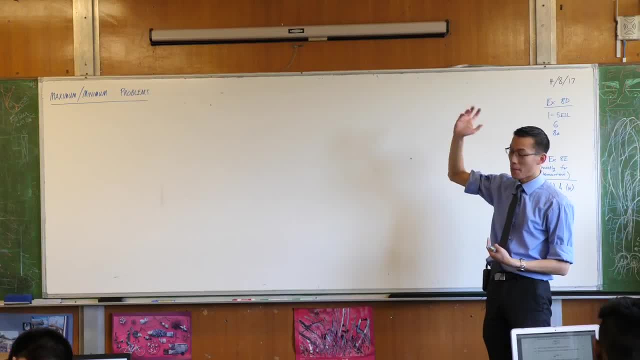 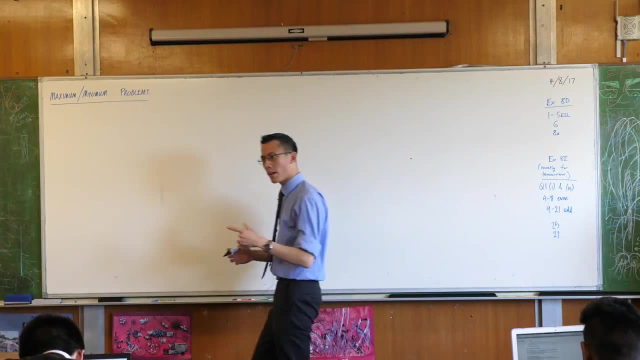 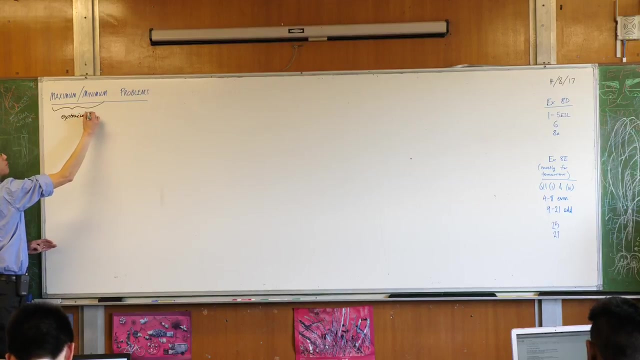 All those kinds of things are an area where basically, mathematics reigns supreme. So max-min problems are a highly practical thing. As an overall umbrella we often call these max-min problems. In the real world we call these optimisation problems. So the idea is: we're doing. 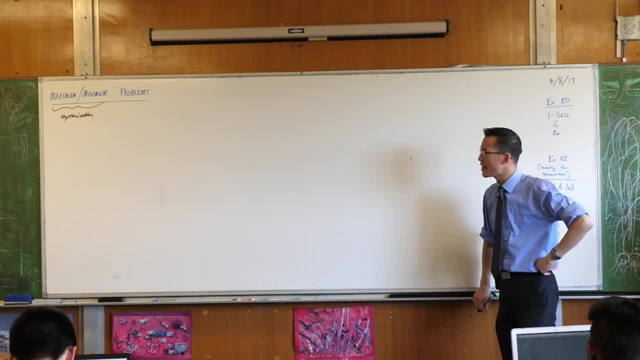 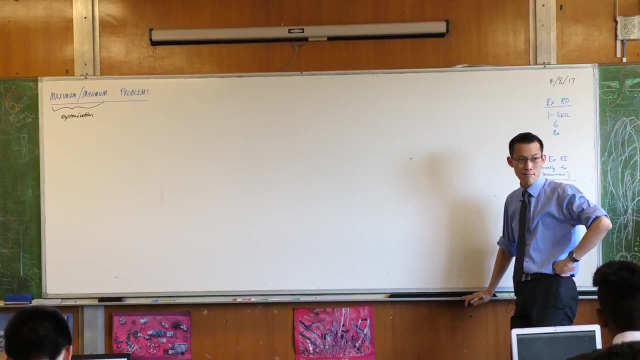 We're doing things right now in a way that's: eh, it's okay, but I think we can make it better. I think we can get more profits out of this even spending the same amount of money. Or I think we can get the same amount of profits but spend less money. 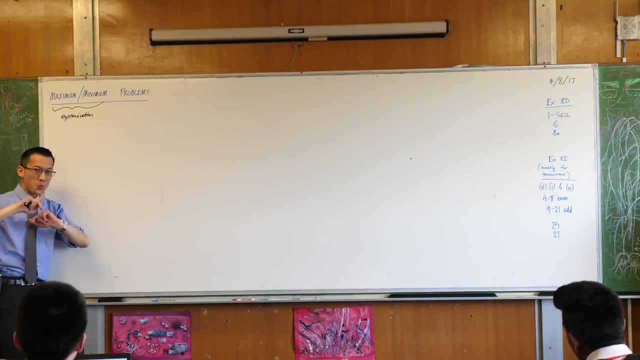 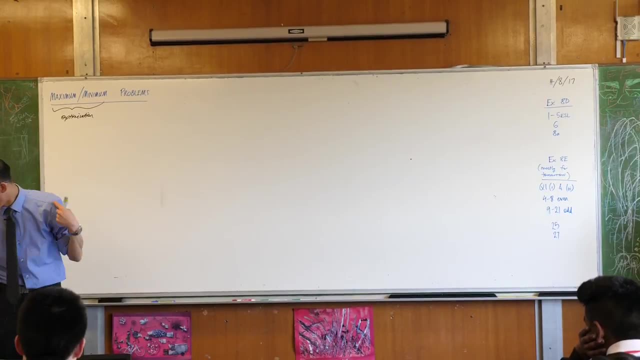 We're trying to optimise, we're trying to improve the situation. The reason why we particularly care about these within quadratics is because they're so very easy to find. They're so easy to find Underneath this heading. draw for me just a quick set of axes. 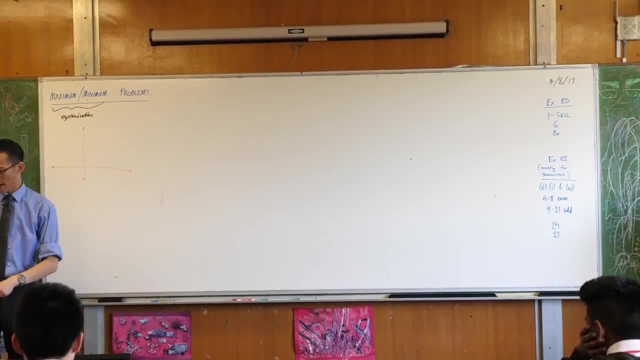 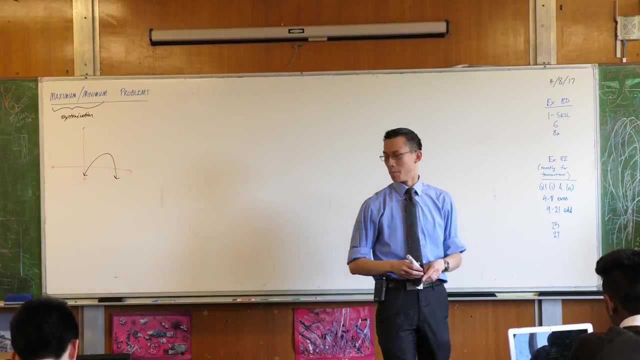 and it's very easy to illustrate the fact of how easy it is to find a max or min when what you're dealing with is a quadratic function. So here's a parabola. It doesn't have a minimum Minimum. saying minimum doesn't really make sense here, because it goes down forever.